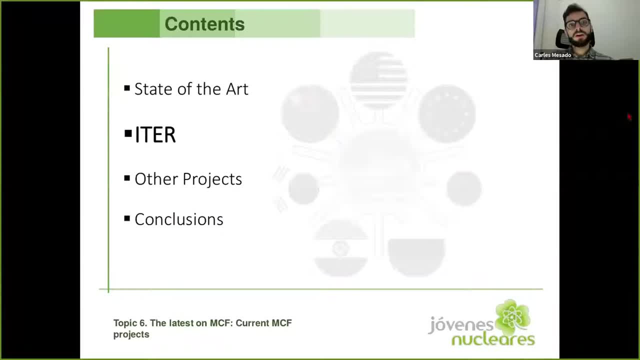 Okay, so after this video, you for sure will know what ITER is about, because it's the main topic here, as you can see. But first I would like to summarize a little bit what we saw the other days, the two previous days. 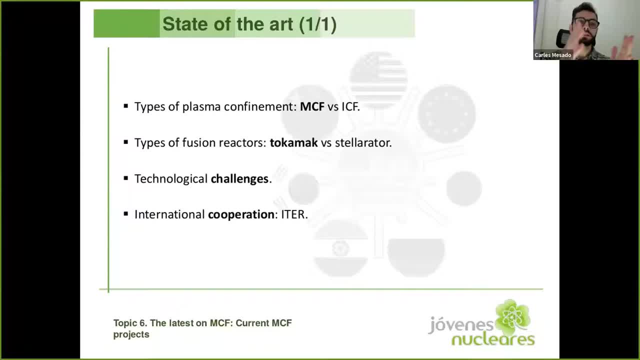 So for confinement plasma we have two main kinds of confinement magnetic: MCF and inertial ICF. We're going to talk about magnetic in this video presentation. For magnetic, we have two main kinds of reactors, That's the tokamak and the stellarator that Enrique talked yesterday about. 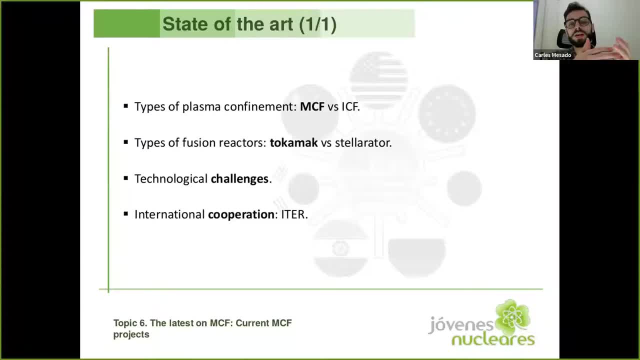 Let's say the scientific community has more confidence or more experience in tokamaks. So that's we are going to focus here today. But any technology here for fusion, we are going to face a lot of challenges. Raquel told us yesterday about these challenges. 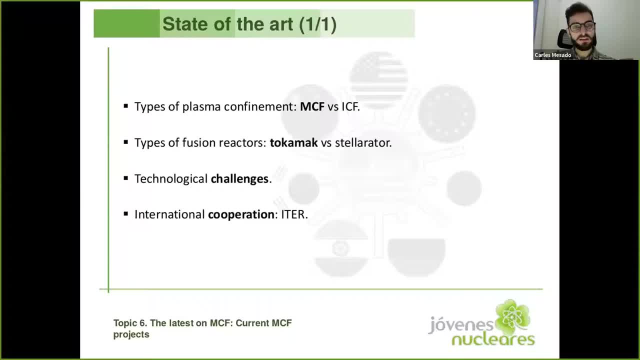 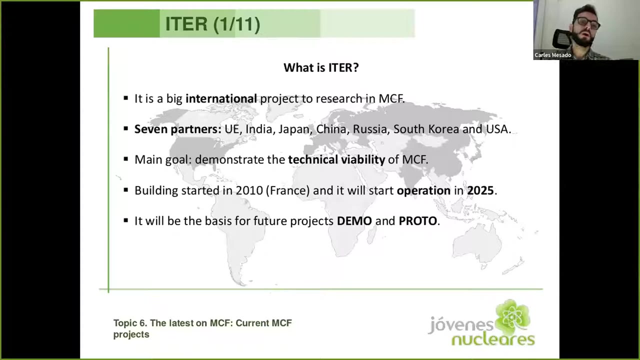 But they are really important in scientific community. But to face these challenges and to overcome these challenges, of course we need international cooperation, And that's where ITER project comes into the play. So what is ITER? If you don't already know? ITER is a project. 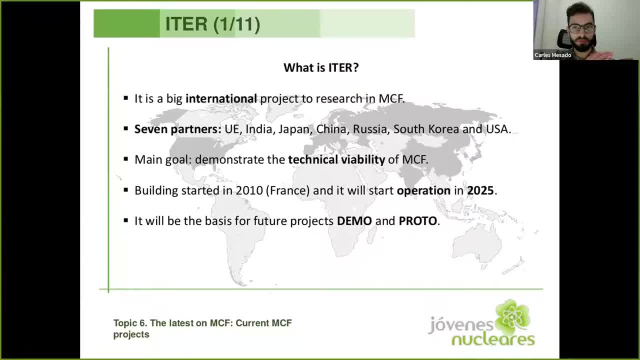 It's a big international project to research on magnetic confinement fusion, or MCF- Only magnetic in this case. It's composed by seven partners, especially the European Union, but also India, Japan, China, Russia, South Korea and, of course, the USA. 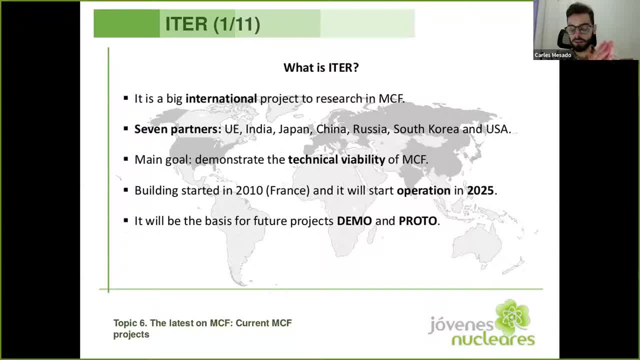 The main goal is to demonstrate the technical viability on magnetic confinement. The main goal is not to produce electricity or energy for commercial purposes. It is only to develop the technical viability. The building started in southern France in 2010 near Cadarache. 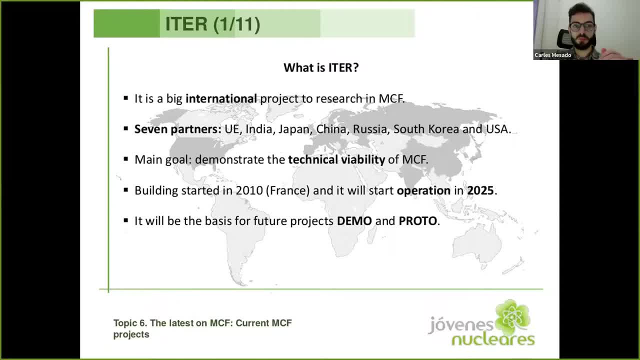 And it's supposed to start operation around 2025, we hope. However, this is the first step in a ladder towards the final fusion power plant. So the first step is ITER, Then it will come a demo And finally PROTO. 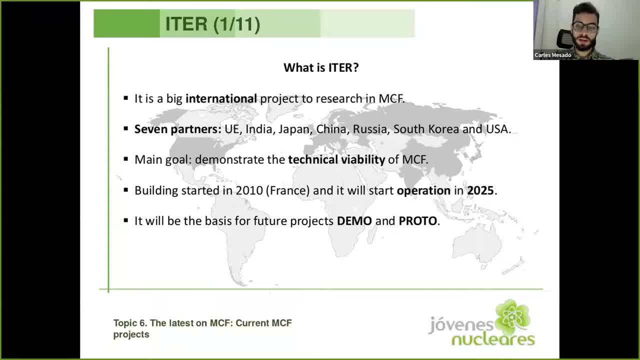 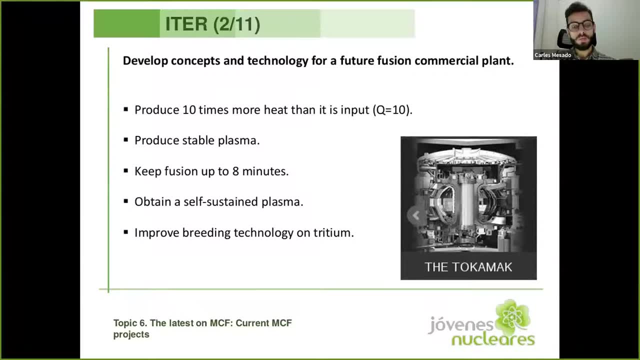 This PROTO will be the first fusion power plant, and commercially, of course. So if we dive into the main goals for technology, we want to produce 10 times more heat than with this input. That means we want to produce 500 megawatts. if we introduce 50 megawatts, 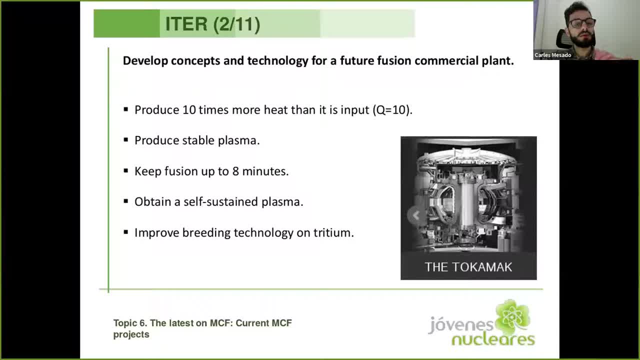 We want to produce stable plasma. As we saw yesterday- I think Raquel explained to us that it's kind of easy to obtain an instability. We don't want instabilities, but we know it may occur, So we must learn how to control them. 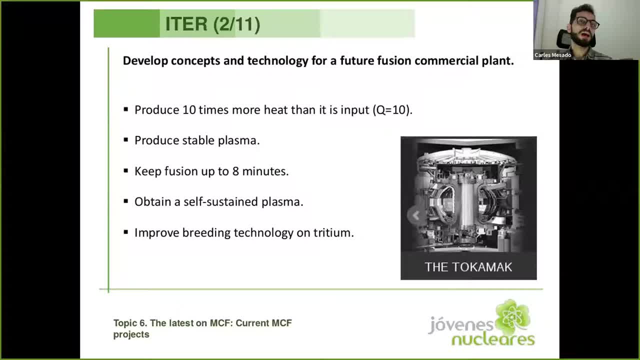 We want to keep fusion also up to eight minutes. That may be not a lot for you, but I must tell you that the biggest tokamak reactor in operation is CHET, which is in the UK. It can hold fusion up to one or two minutes maximum. 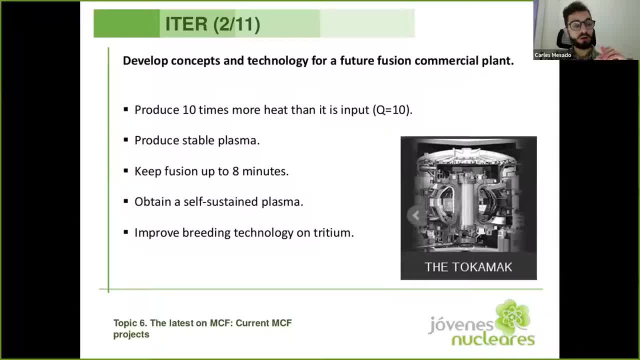 So it's quite a lot, eight minutes. We also want to obtain self-sustaining plasma. That means that initially, in the first stage, we need to supply heat to the plasma. However, at a certain level, the plasma should keep moving on by itself. 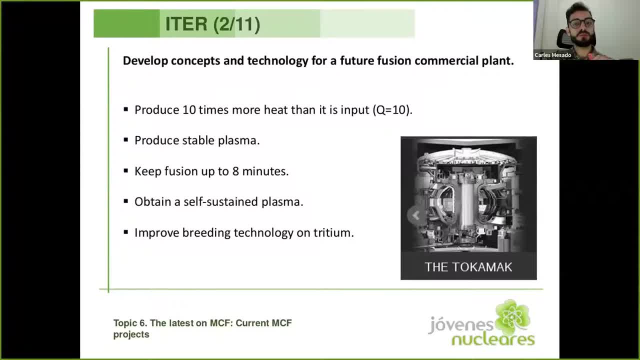 So it is self-heated, let's say. And we also want to improve the breathing technology in 3D. So those are the main goals in the technology we want to develop. We already see this picture hundreds of times if you are into fusion. 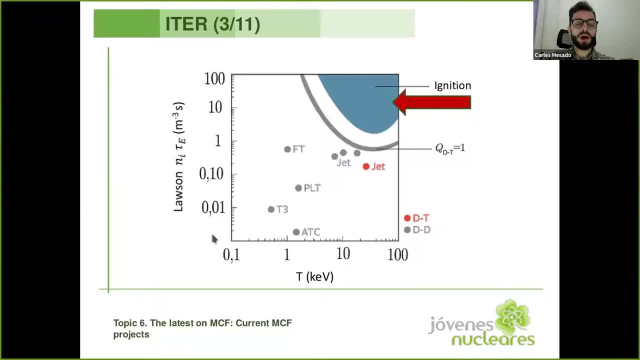 But I want to show you it again. These points represent the reactors that are in operation nowadays. As you can see, CHET here is one of these ones. It's the main, the biggest tokamak in operation, And we want to do a jump and go into the ignition zone. 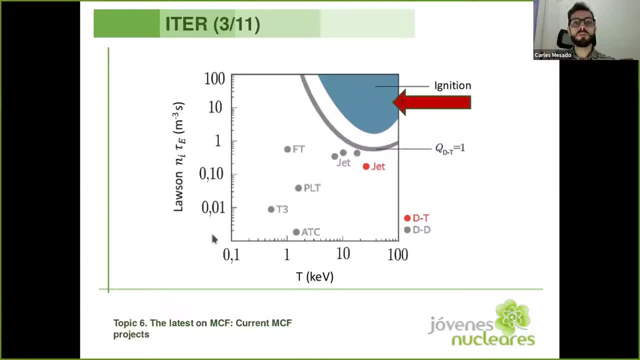 The ignition zone is the blue area And ITER will be here around here where the red arrow is pointing. So of course you can see that both axes are logarithmic. So you can imagine that this is a giant jump because both axes are logarithmic. 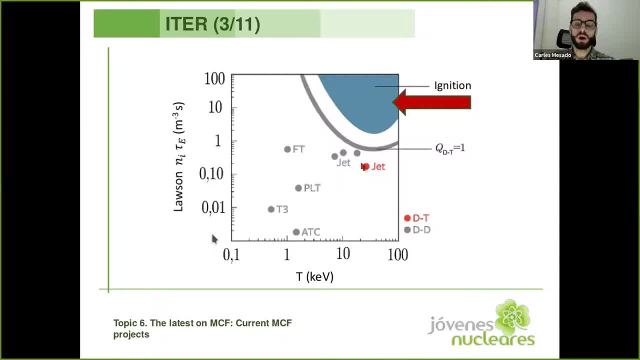 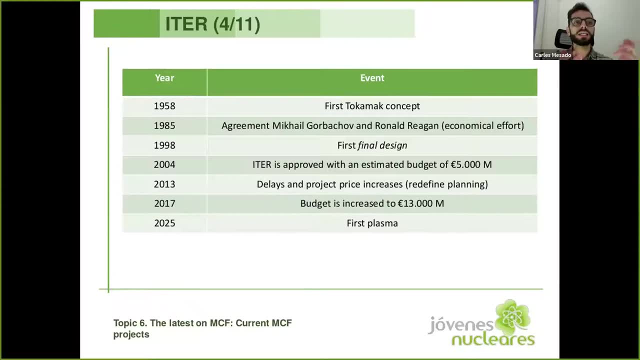 That's where all these challenges come from. But we must overcome these challenges. So I want to talk about a little bit. what's the story behind us that led us today here to talk about ITER. So it all started in 1958, where the first tokamak concept was presented. 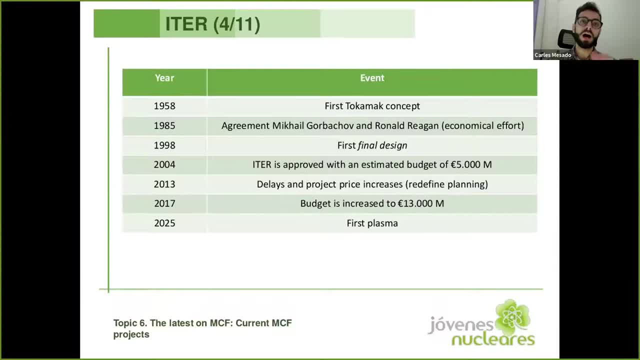 It was presented in a conference, the second conference of Atoms for Peace. It was presented in a paper. This paper was presented by a Russian scientist called Vladimir Mukhovatov, And of course he is working at ITER. He's the equivalent Messi for fusion. 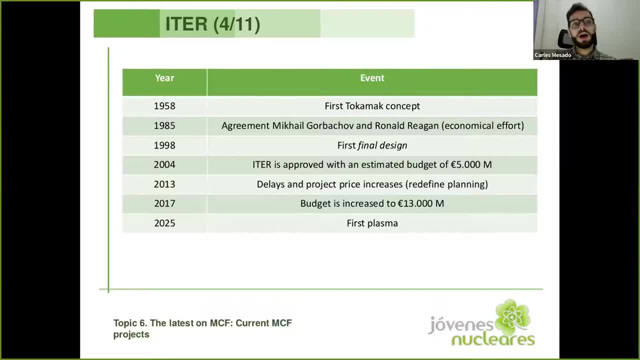 Of course he must work at ITER Afterwards in 1985, the more important people on Earth at that time, Sergei Gorbachev and Sergei Reagan. they bring together an agreement And of course this agreement was built because of economic effort. 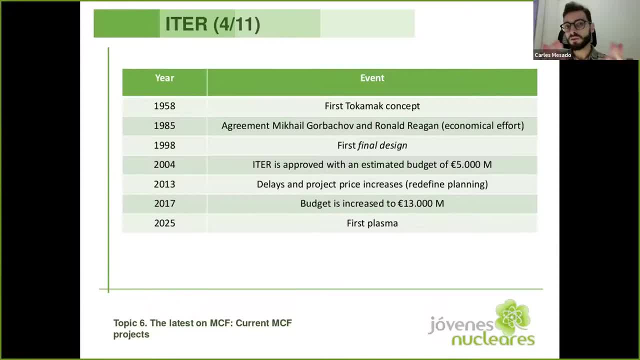 This agreement was to develop fission for civil purposes And this agreement was made because they didn't want to spend all the money alone. So they need to join forces. let's say In 1998, we had the first final design. 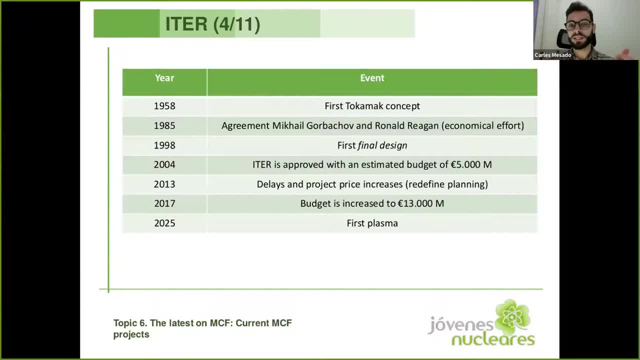 And final design is in italics because we have several final designs. as we will see, In 2004,, ITER is approved with an estimated budget of 5,000 million euros, But of course we have delays In 2013, because we want to introduce the technology. 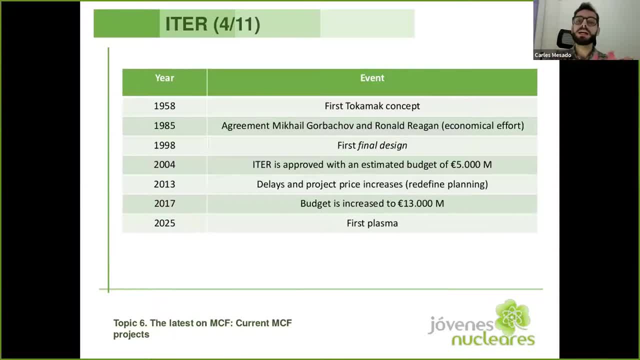 because in all these years the technology advanced. there are new materials, new simulation codes, new projects etc. that we want to introduce in our ITER project. So there are delays and we need to increase the budget. We increased the budget in 2017 up to 13,000 million euros. 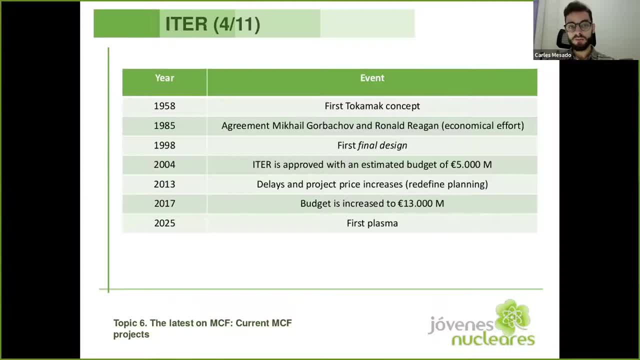 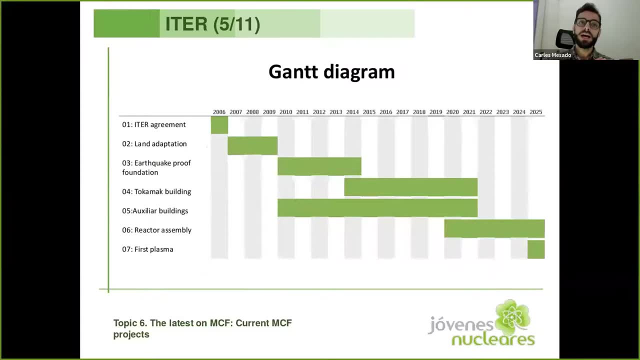 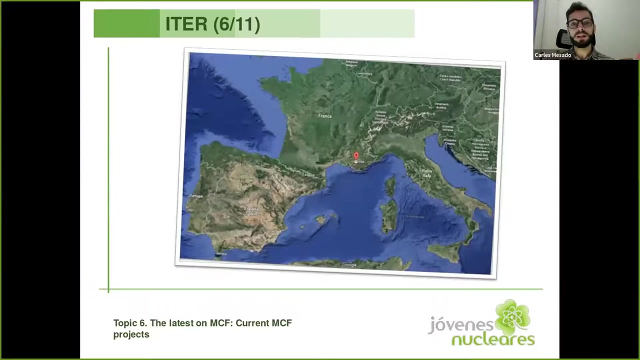 We expect or we want to obtain the first plasma in 2025.. Here you can see a GAN diagram for the main milestones in this project. We are around here, So mainly we are starting building the reactor And we are going to see pictures of the real site, the real ITER project, the real reactor. 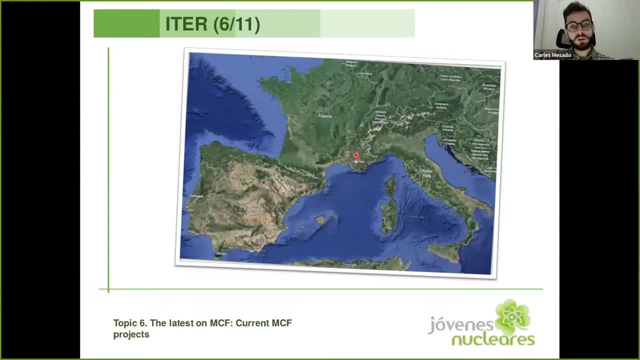 or what we have right now at least. So, as I told you, this project is being built in southern France, near Cadaraz. Of course, there is good weather, good wine, good food. We zoom in, We have this area. 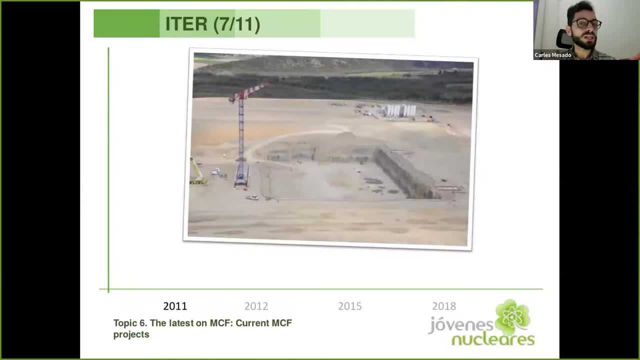 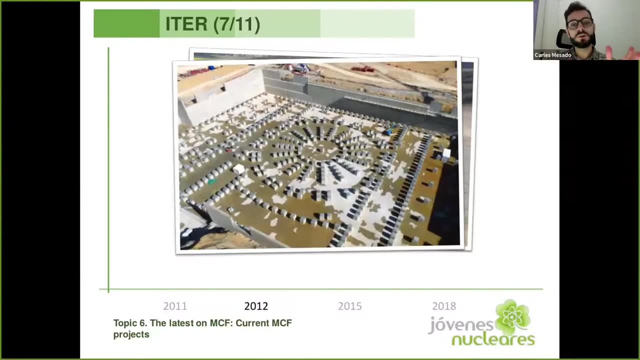 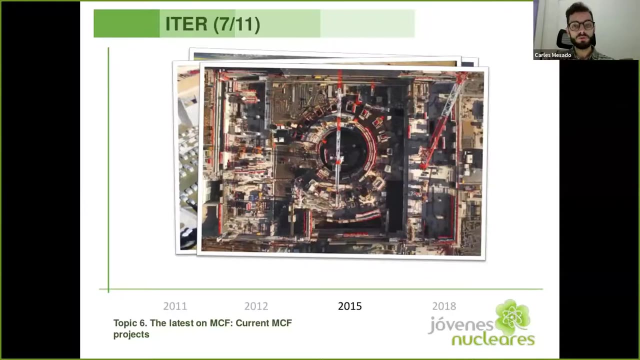 In 2011, it looks like that It was not really promising: just a hole in the ground, but something. Then, in 2012,, we have this: These cubes are the earthquake-proof foundations. In 2015, we have this nice picture from the sky. 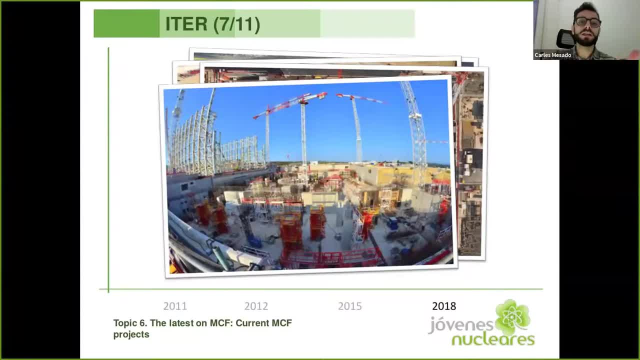 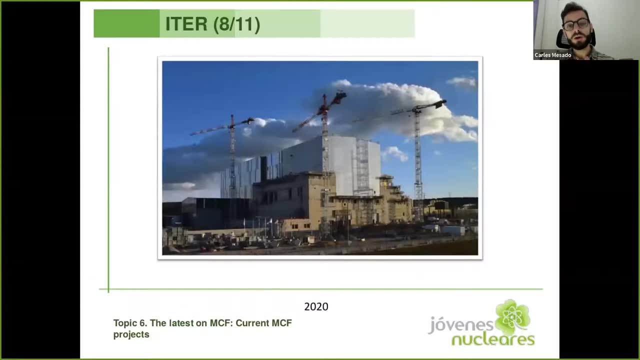 In 2018, we have this. It's starting to build something, And you may ask yourself what it looks like today. So we are going to see it. This is a picture. This is how it looks like today. This is the main reactor building. 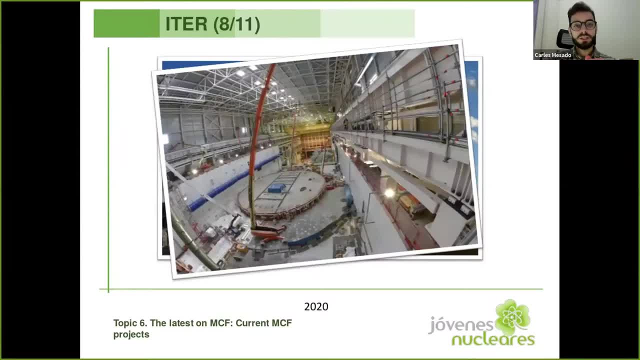 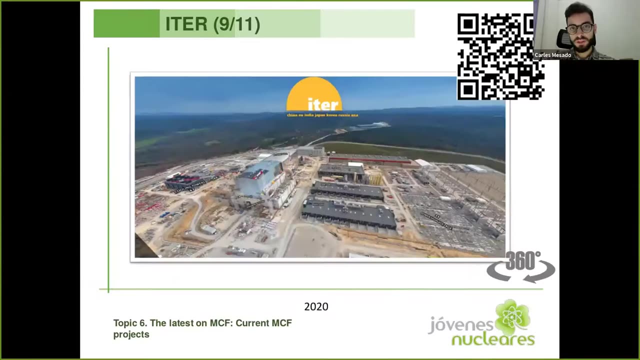 And we are going inside the reactor building. So this is the main hole And under these lids it will have the reactor, the real reactor. We remove these lids, we have this hole. That's where the cryostat will be. 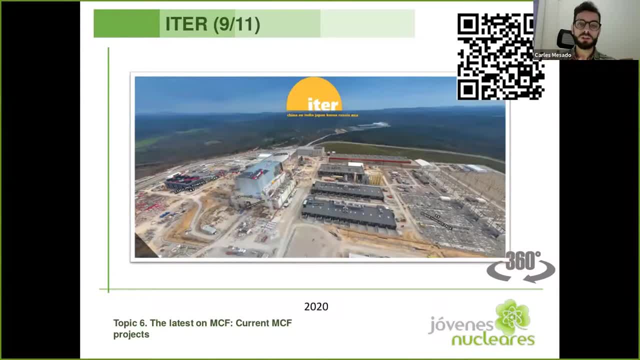 And for those of you who like to see the things by yourself, I know you can visit this facility by yourself. However, I understand the wait on this is quite long, So I invite you to go to the web page or to scan the QR code. 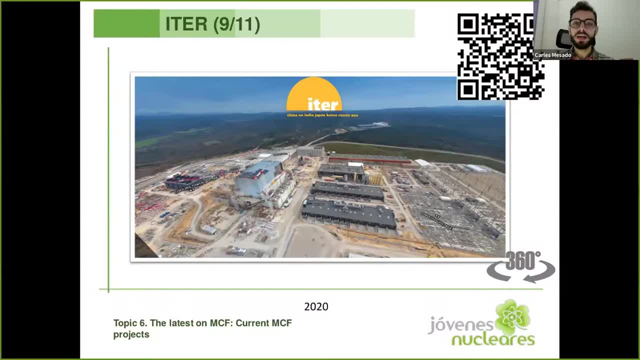 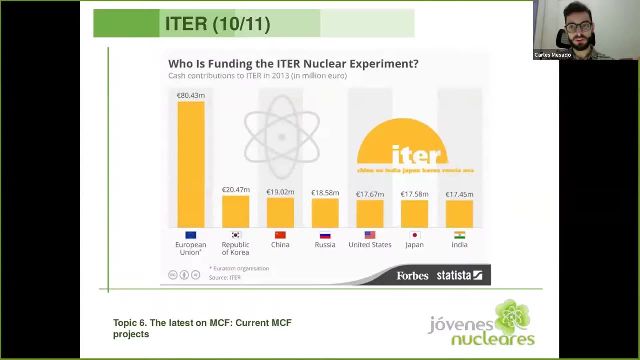 So it will take you to a virtual visit And I really enjoy it. So I really recommend you. You can visit several buildings, several parts of the facility And, of course, you can move through the axis of time. Another important question you might ask yourself is: who is paying all of this? 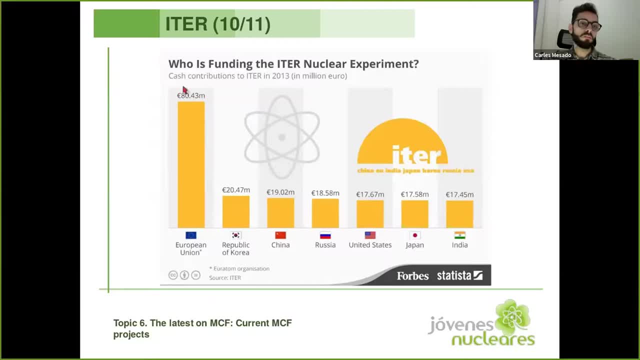 So, of course, we are a European university. We are a European university And we are paying most of the budget. This is an example for 2013 in million euros. The European Union was paying 80 million euros And the rest of the partners- the other six partners- they were paying each one around 20 million euros. 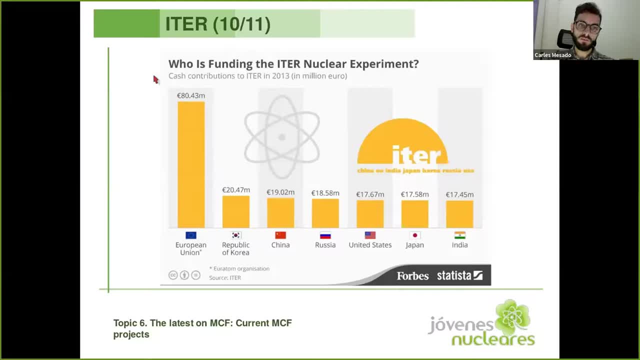 Yes, we pay the most, But of course we also get the most of the benefits. It's not a coincidence that we get the reactor in France And in Spain And in southern Spain, Granada will get an experimental facility or laboratory to advance in materials for fission. 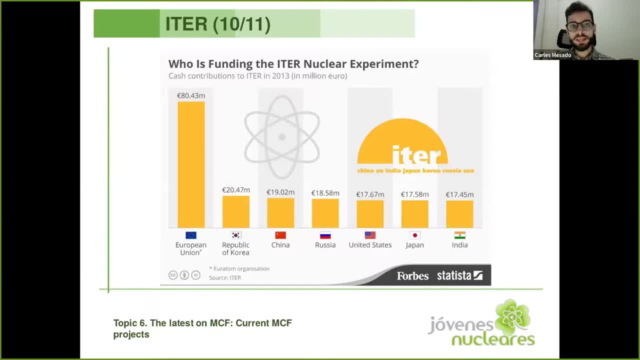 I hope we get that soon. That may be a lot- 80 million for you if we compare that amount of what we have in our bank account, But I tell you it's not a lot for these countries or for the European Union. 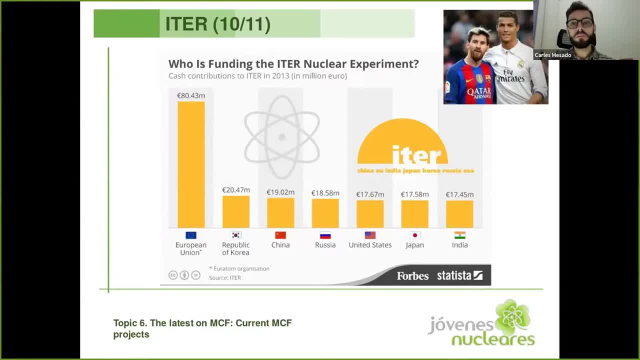 We can compare these amounts with what the income for Messi Barcelona football player, or the income for Cristiano Ronaldo football player. Both of them have an income of around 30 million per year, So that's not really a lot. So if they are watching this video, I invite them to support this project with their income. 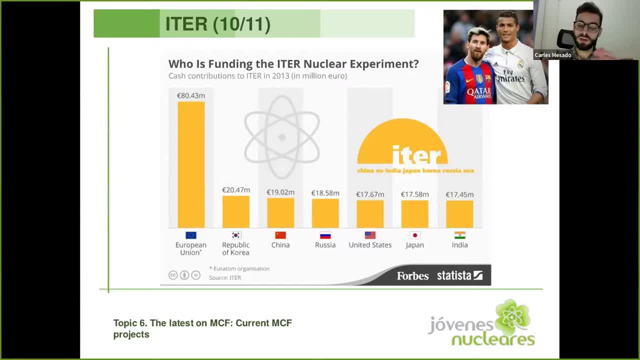 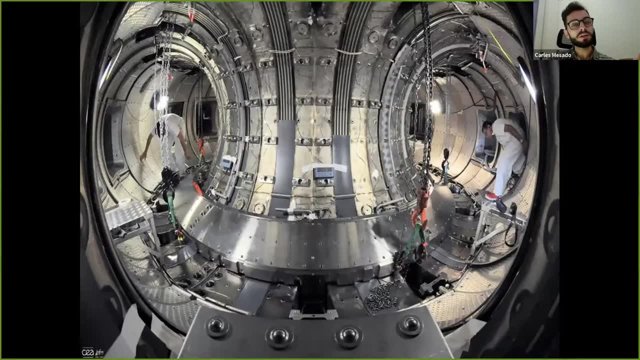 If they do that for several years, we will have this reactor really soon. I hope so. they are watching this. In this picture you can see the vacuum vessel. This is not ITER, because, remember, ITER is being built. This is JET in the UK. 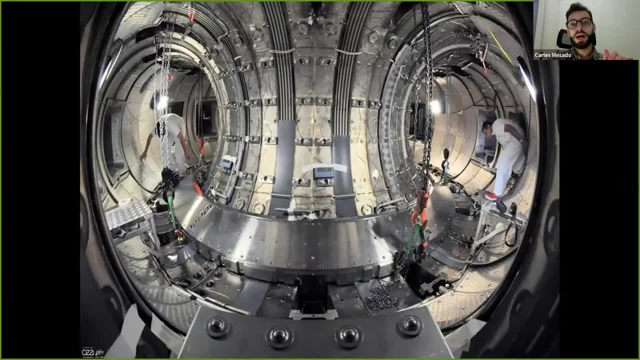 Which is the biggest tokamakin operation right now, And because we have two men, we have a reference, We have an idea of what's the real size of this vessel. In ITER this vessel will be around two or four times bigger. 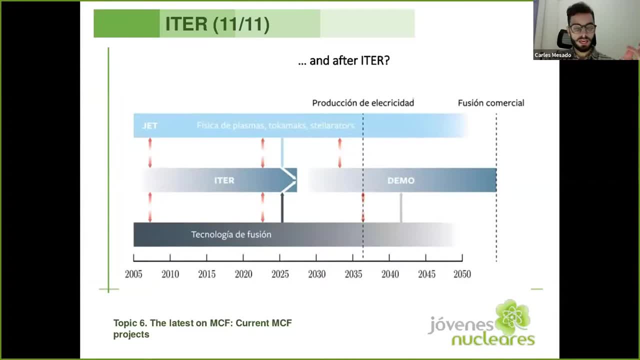 So what about AFLUR ITER? As I told you, this is the first step in a chain of steps. The first one is ITER, Then we'll have DEMO And finally we'll have PROTO around 2050.. And that will be the first component. 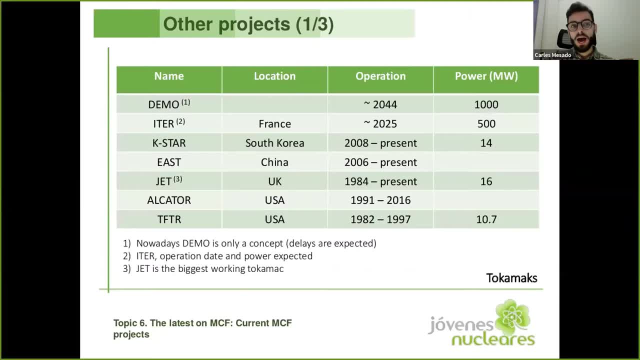 This is the commercial power plant by FUSION. Before ending this presentation, I would like to talk a little bit about other projects. In this table I summarized most of the tokamaks in operation. I would like to focus right now in JET, which is the biggest tokamakin operation. 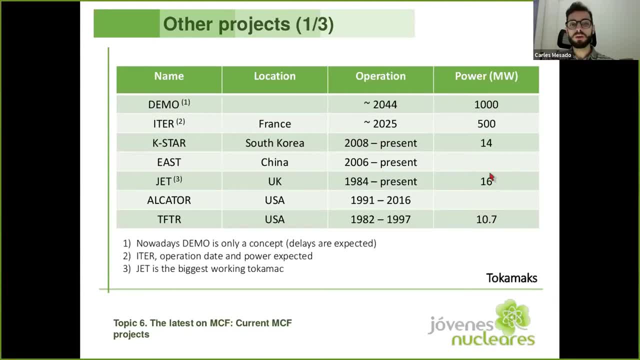 It has a power of 16 megabytes And we want to jump in power up to 500 megabytes to ITER And then DEMO 1000 megabytes. So you can see the jump is quite a lot For stellarator. I have the same table. 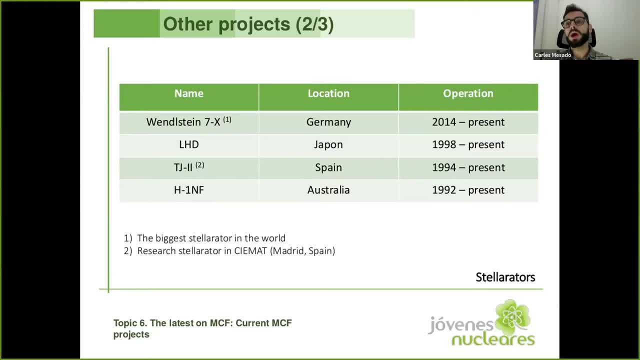 You can see there are less stellarator in operation. That's why we have more experience or we are more confident in tokamaks And that's why we choose a tokamak for ITER. I want to focus first on the first one, the German, which is the WELSTENSTEIN 7X.